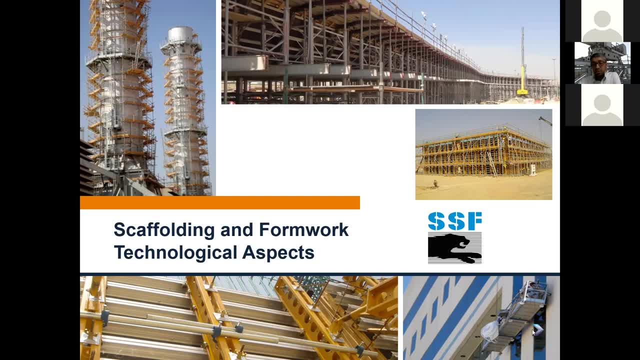 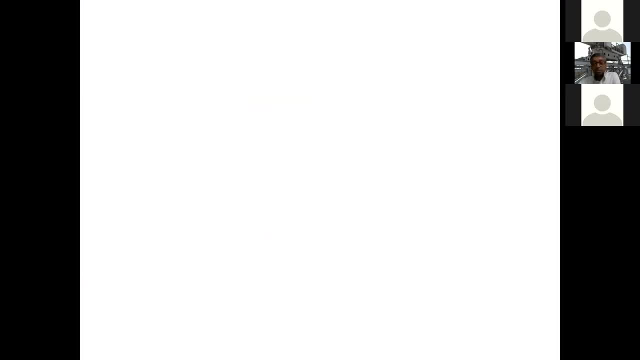 So let me start with this. So let me start with a small introduction. Basically, this will be an interactive section. You can stop it anytime if you want, Or you can ask questions anytime. I will ask you a question as well, All right. 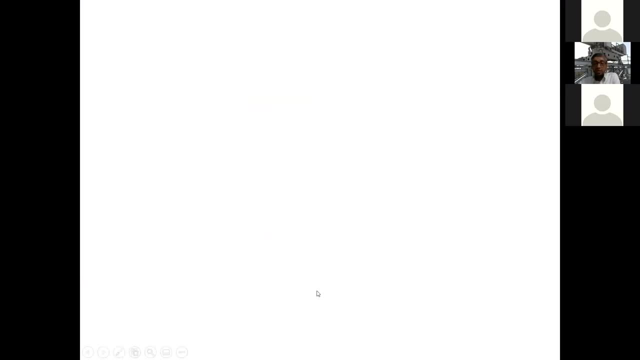 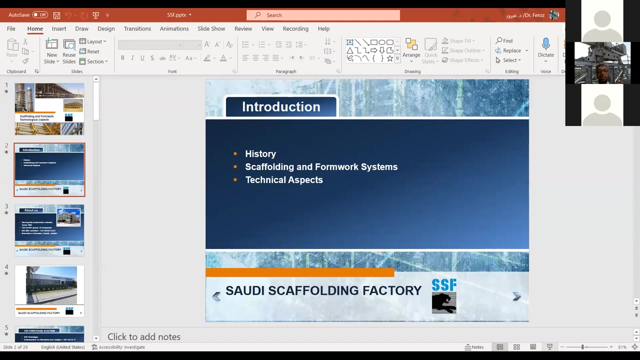 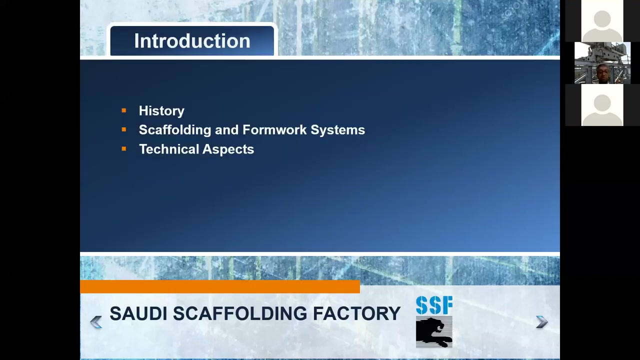 Okay, Can you see the next page? Still not showing but I think probably still loading, Taking time, Can you? Hello, Yeah, we can see it. now We can see the slides. Okay, So I'll start with a brief introduction of the history of our company, then we'll move on to the scaffolding system, followed by a formwork system and some brief technical aspects on this. 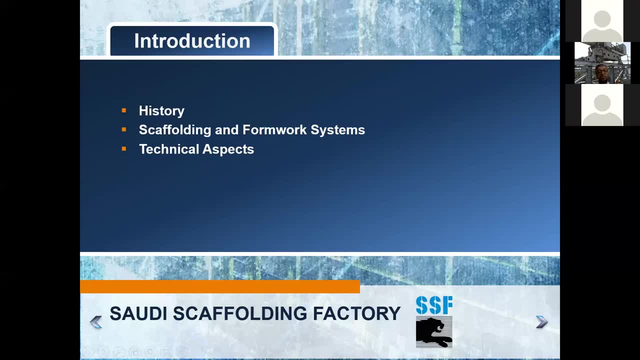 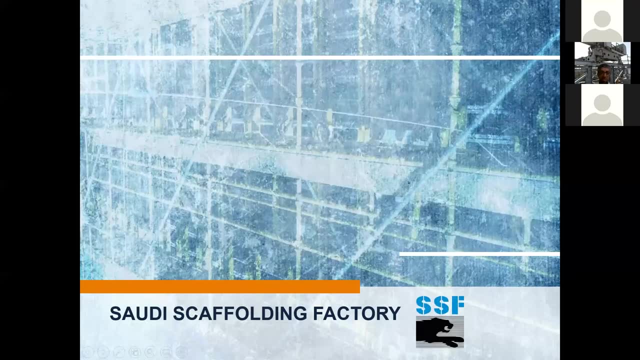 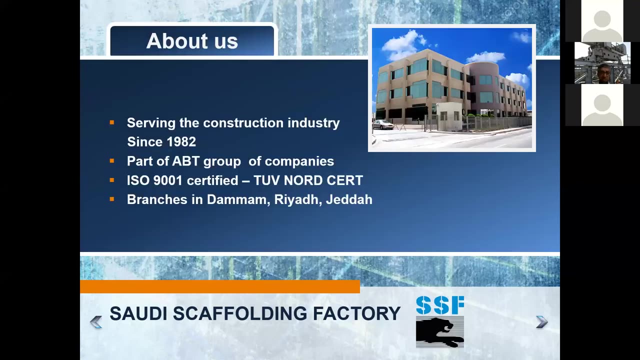 Okay, So this scaffolding company is established since 1985 in this industry, for more than 35 years. We have a factory in the mom and we have branches in the mom. We are basically we cover all Saudi Arabia And we have a good reputation, reputation because we are in a local company. 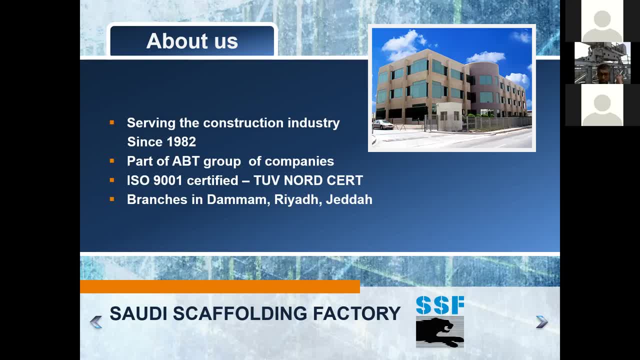 And a lot of prestigious projects: Aramco, Saabek, Municipality. all these projects we have taken completed successfully And we are part of the ABT group, which is located- you know this building, you might have seen in this- in Khober, al-Bustan area, Raqqa. 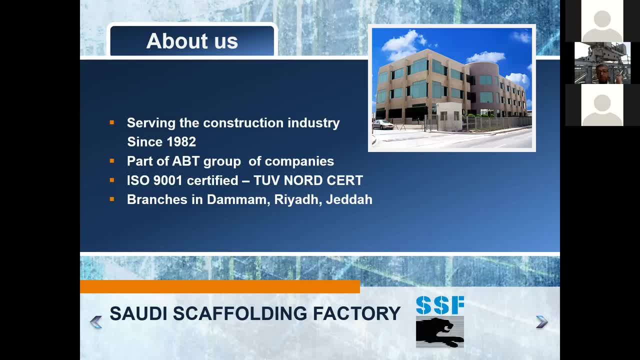 This is also our main company, which they are famous for distribution of cement. We are an ISO 9001 certified company. We have auditing every six months, So this makes sure our quality and safety of the products And it is again one of the requirements for Saudi Aramco and Saabek. 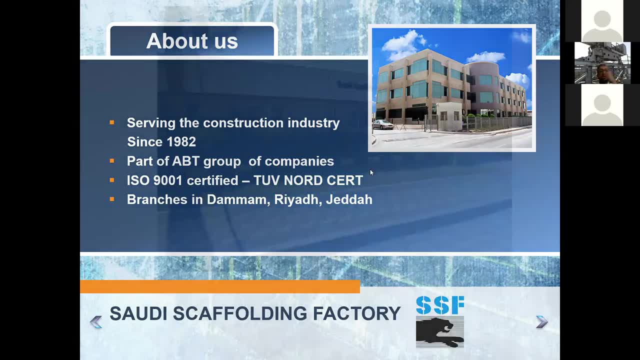 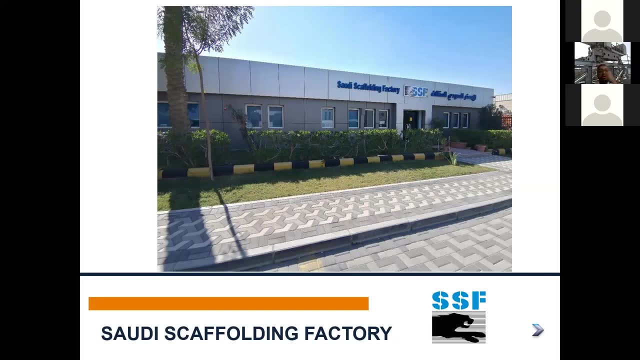 This is our company, Oh, sorry, Our factory. This is our factory in the first industrial area. The look from outside, from the road, what you can see, it will be like this. So our factory is based in the mom, where we manufacture our scaffolding and form of products. 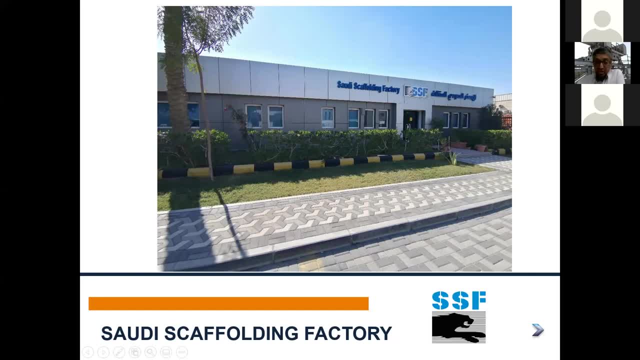 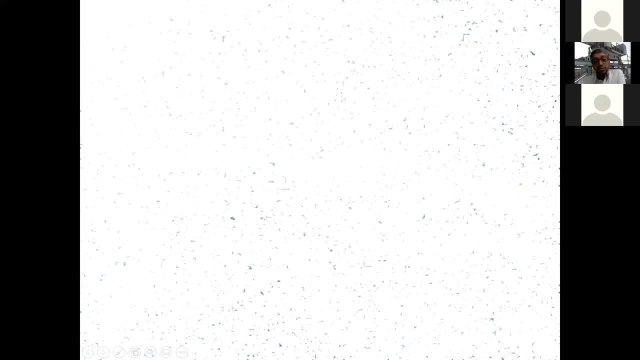 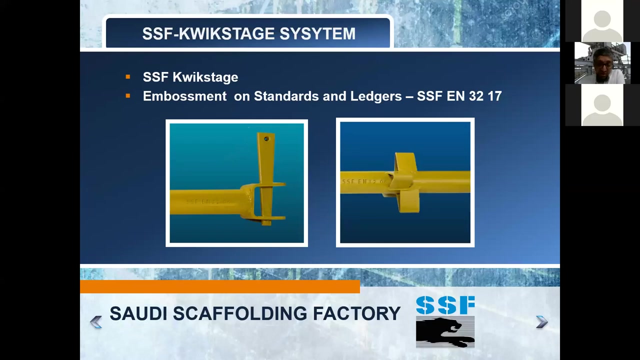 And you know I sit in this office also. We have a design team here in the mom and sorry. in Jeddah and in Riyadh We have different, you know- system for scaffolding. Basically this is a pipe or tube or circular hollow section- you know the terminologies I'm saying- fitted with some connecting components. 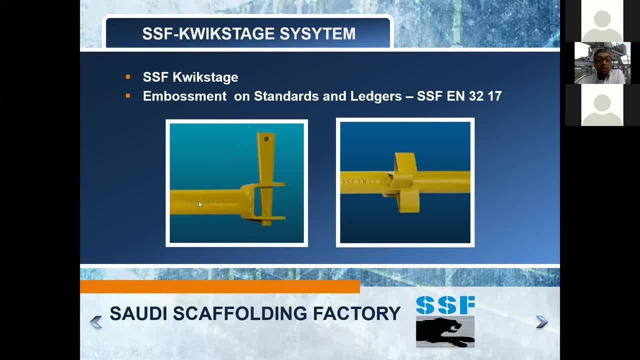 The one on the left, you know, it's called ledges, And one on the right is called the standard. The ledges are horizontal members, whereas standards are horizontal. The ledges are horizontal members, whereas standards are horizontal. The ledges are horizontal members, whereas standards are horizontal. 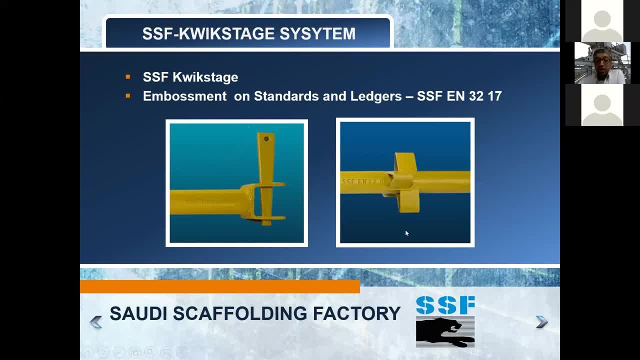 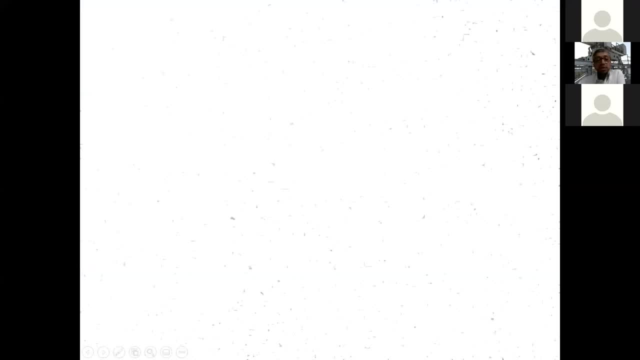 Vertical members And these systems are approved by ARAMCO. And these systems are approved by ARAMCO And there are some specifications. ARAMCO's Whale 2 follows standards And there are some specifications. ARAMCO's Whale 2 follows standards. 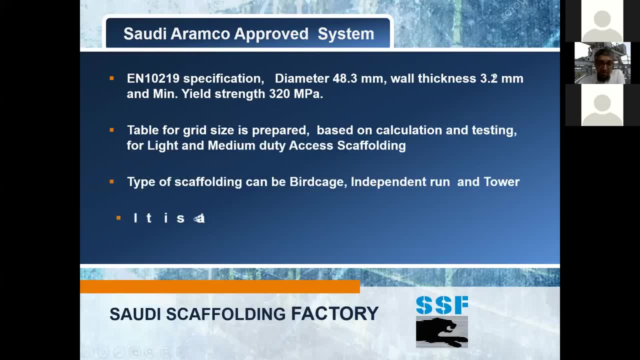 in 1, 0,, 2, 1, 9, and the diameter should be around 48.3.. And the diameter should be around 48.3.. sorry, and based on you know, we have to do some calculations and prepare some grid sizes for the. 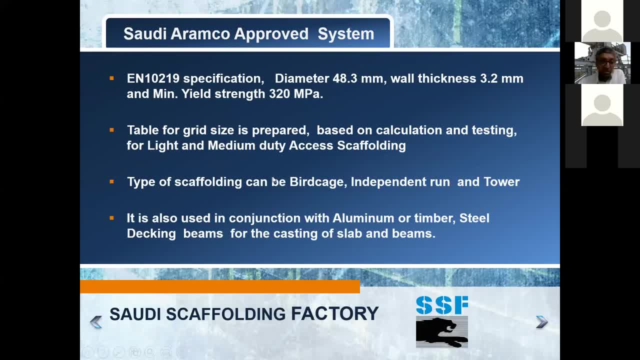 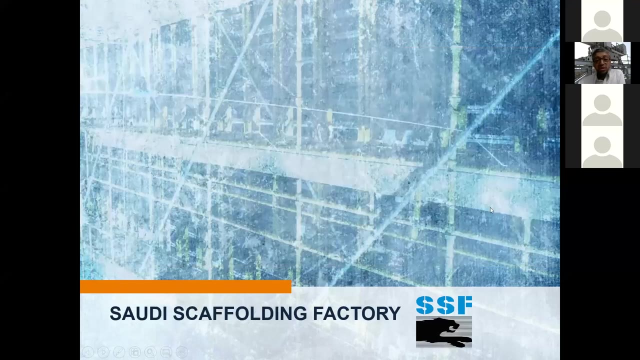 particular load of light duty or medium duty. this is actually, you know, this is a part of what i'm saying- about scaffolding, and then there are different types of scaffolding which i'll explain you with the photos. then you'll have a better understanding. as you can see now, these are the different system of scaffolding we use. this first one is the bird. 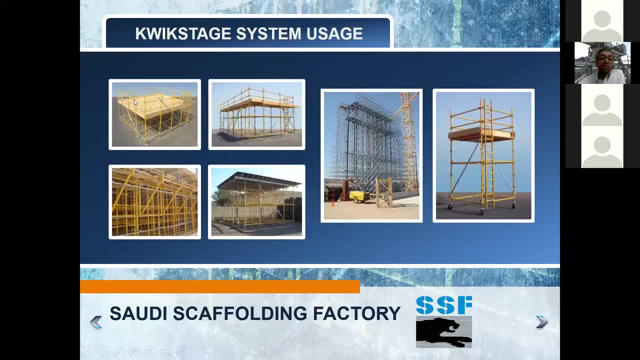 cage where you have. we can work it on, work on the platform, uh, on a big area, and then the other next one is independent run, which is, you know it is uh. if you want to work on on a linear area as well, like that you know we have, you can see a big structure here which we are simulated for. 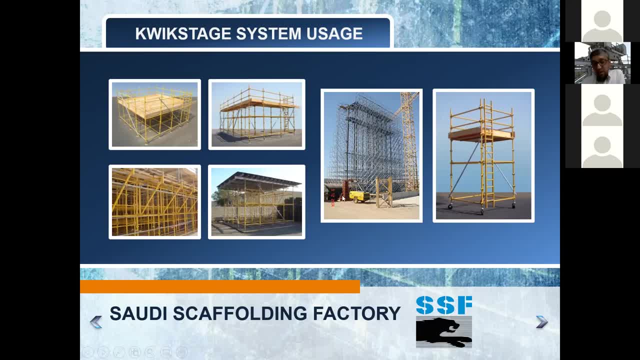 simulated for uh tunnel sewer in mecca and similarly this system can be used as a shoring, which is, you know, as a slab support or a beam support like that. in that one, you know, we. i briefly give you one small video to give a good understanding of uh, how this system works, how this 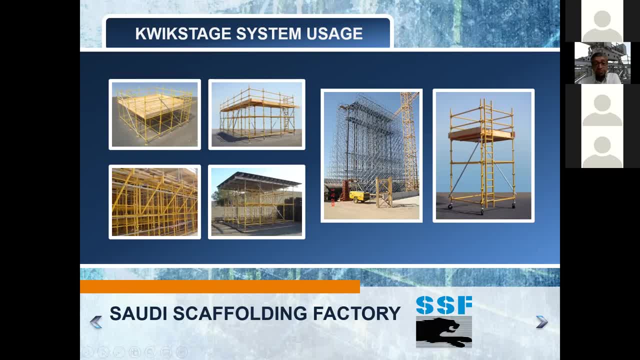 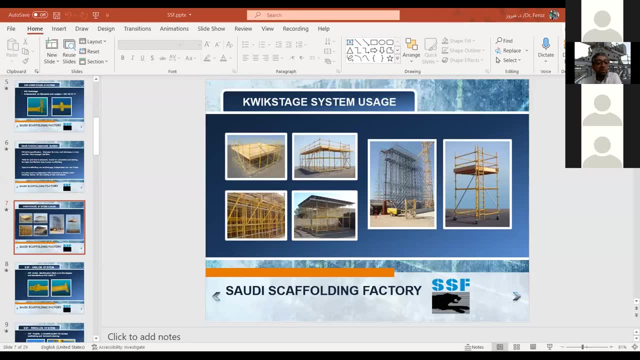 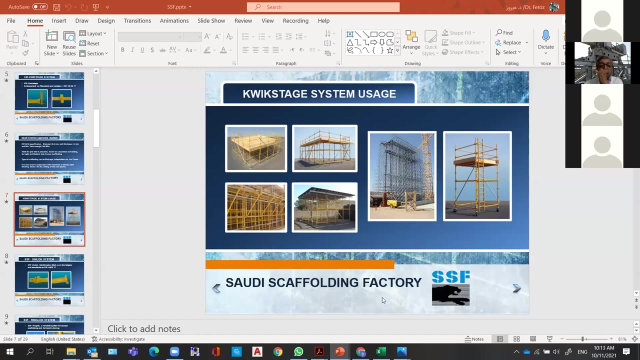 system is in place. Can you see the screen? uh, not yet. we're still looking at the slides, slides um you, j, y, x, h, i, k. It's still not showing. it's a bit slow that way. Is it showing now? Not yet. 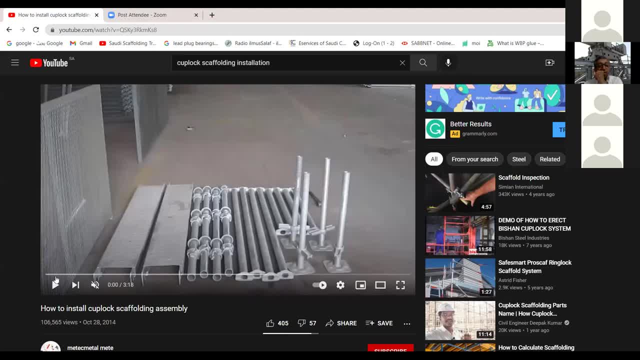 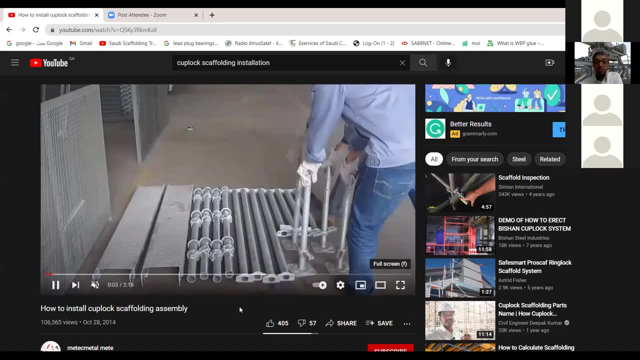 Okay, It's showing now. We can see it now. Yeah, The video you can see now. yeah, Yeah, Yeah, This is how we install. These are called the base jacks, So we'll put four base jacks. 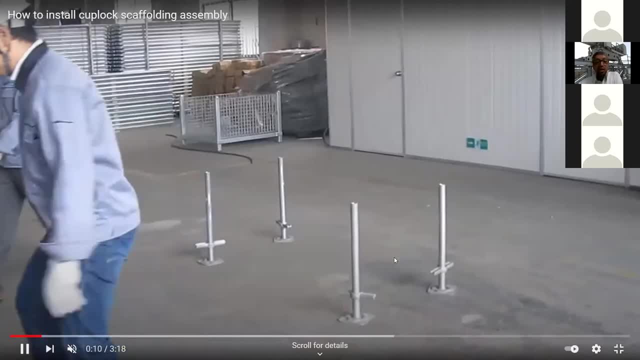 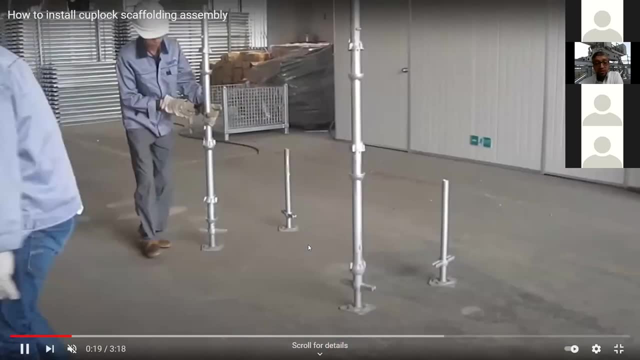 It's clear now, no, Yeah, It's clear, It's clear, Yeah, Yeah, Then they'll put the standard inside the base jack, Base jack. the purpose is to adjust it so that it's not It's leveled properly. 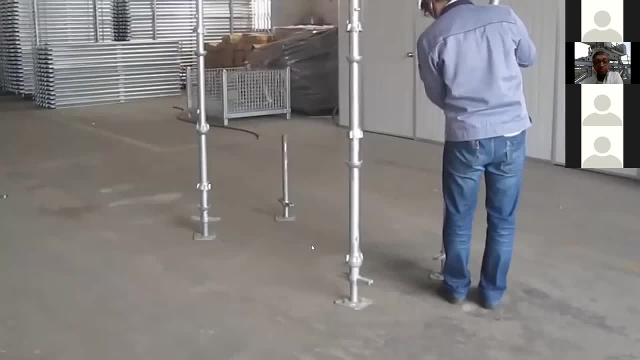 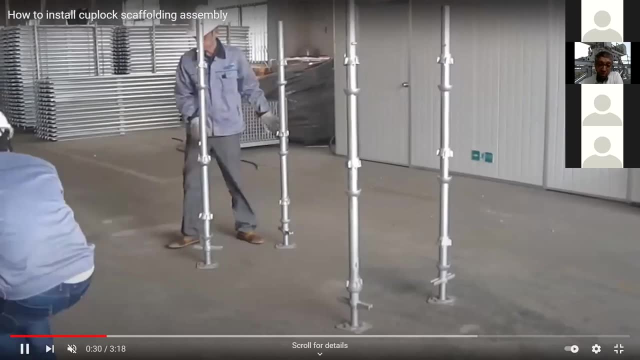 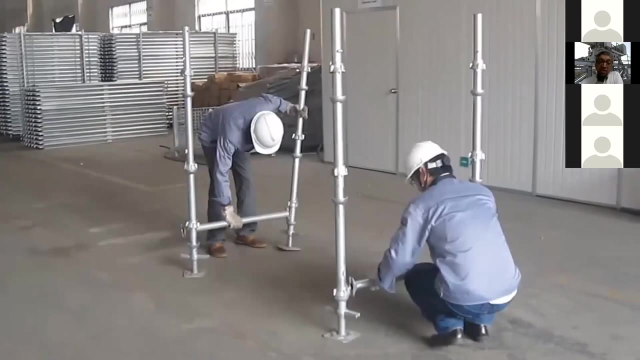 There's no inclination, It's all vertical and horizontal. So this is the component called standard or vertical member, which has some connections, which is called top cups, bottom cups, et cetera. In that top line, between the top cups and the bottom cups, they insert the horizontal. 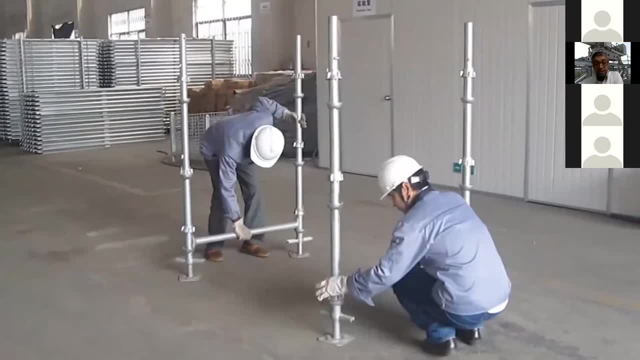 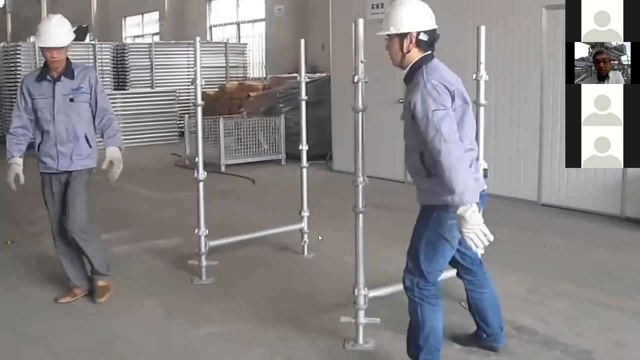 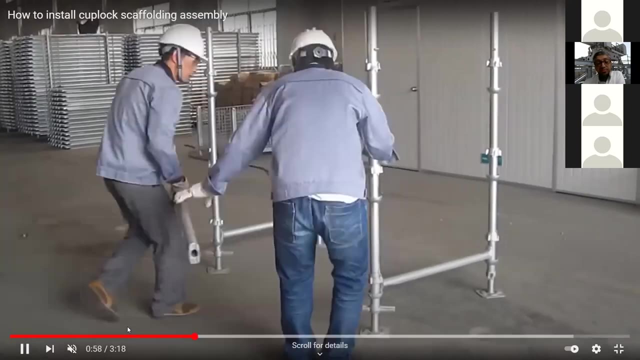 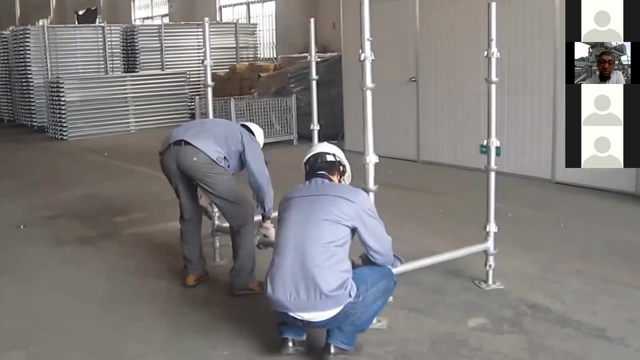 member, which is the ledgers. So once they Inside the ledger- Yeah Yeah, You know, you get one part and like that, they make a frame which you can see And they will tighten it using hammers. 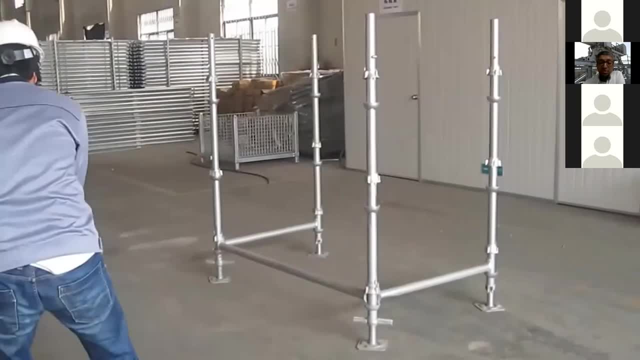 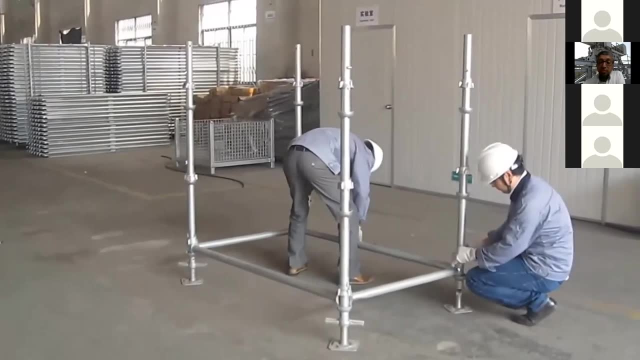 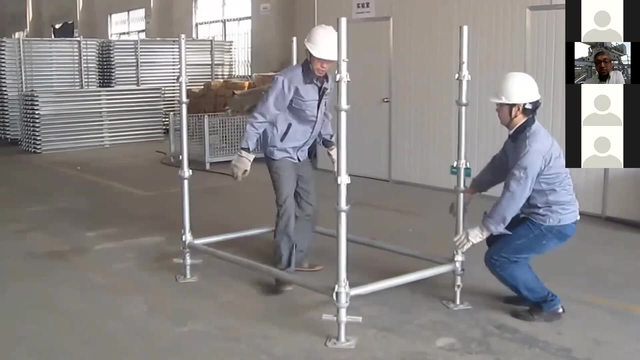 All these are steel members. Like this they form depending on the bracing height. This bracing height and all we will calculate as per the load. What will be the next lift of this horizontal members? Usually, if it's access scaffolding, it will be two meters. 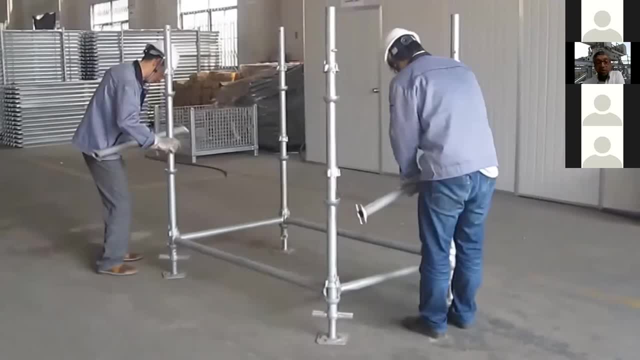 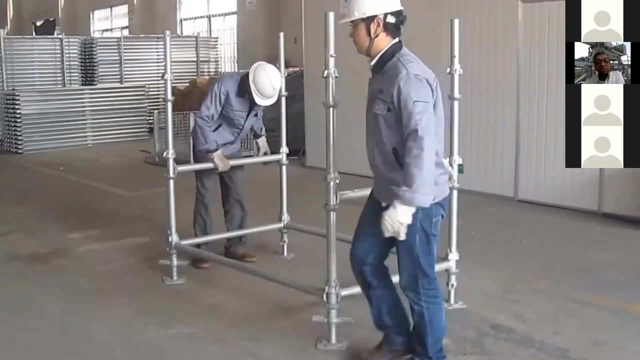 If it's slab support like that, you know heavy loads it can be. We like to put every 0.5 meters These tops, tops, bottom cups. it will come in every 0.5 meters, So you know the maximum height will be. 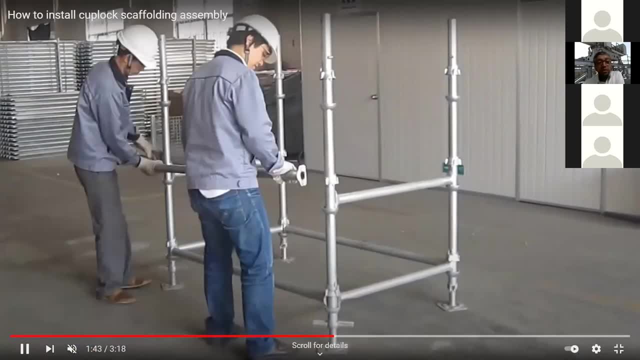 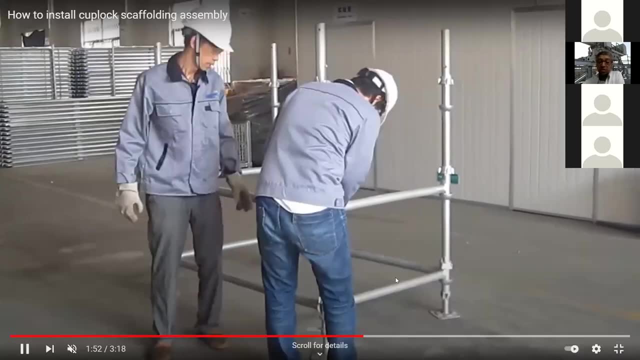 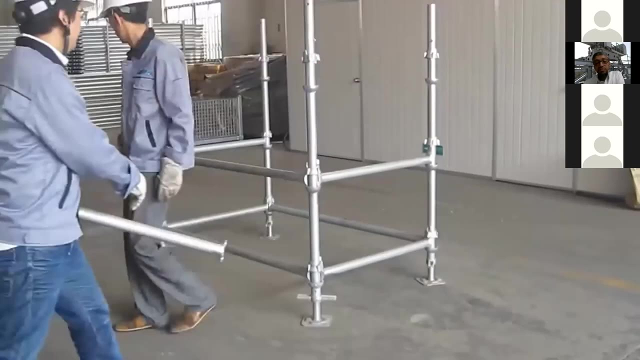 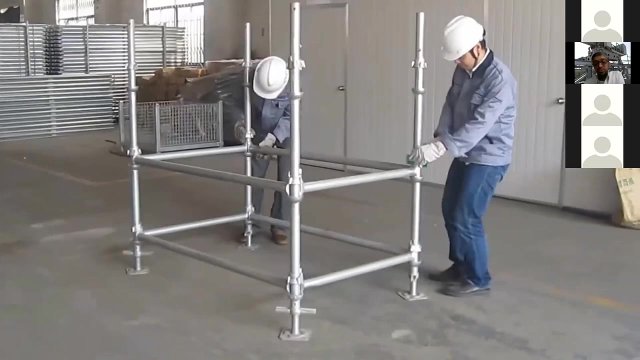 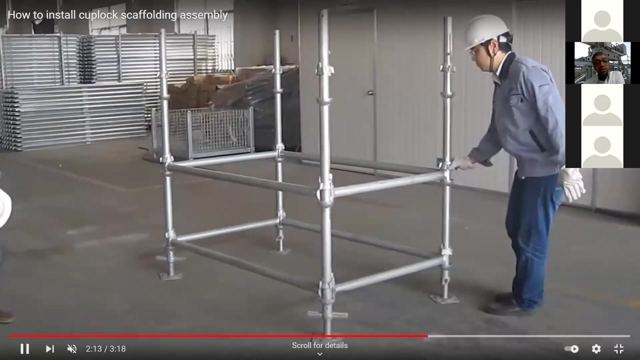 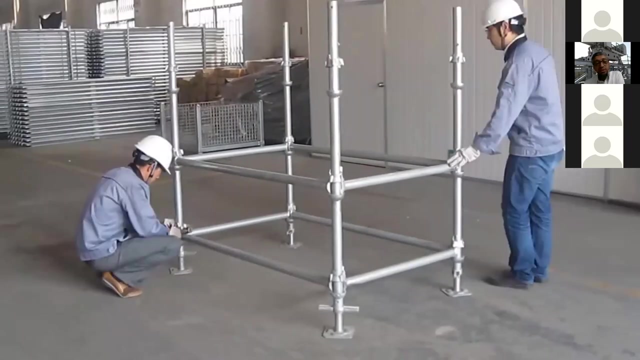 Sorry, the minimum height will be 0.5 meter. Maximum height can be in the multiples of 0.5 meters. Be like this. So this is the members we manufacture it here. You can see it is tightened using slight hammers. 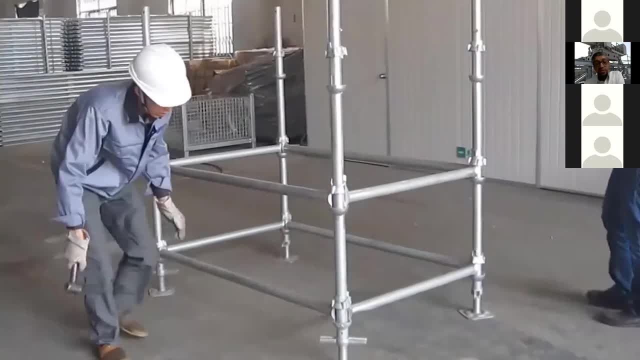 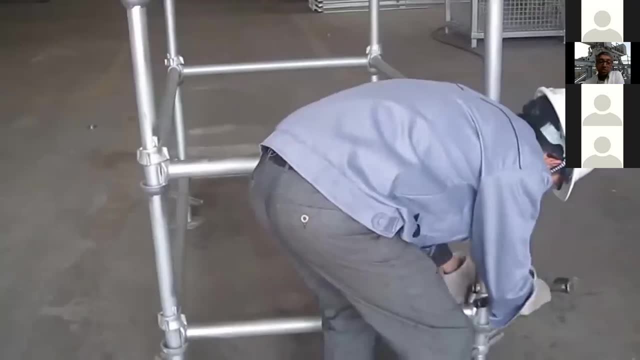 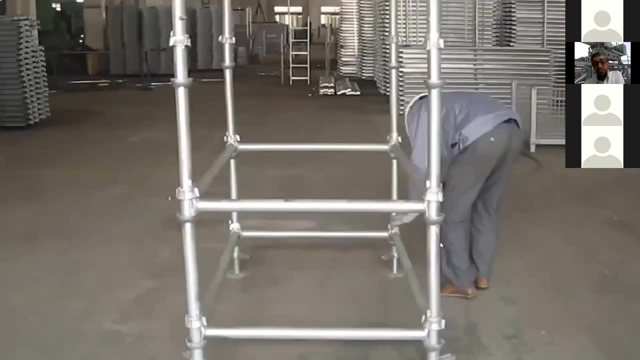 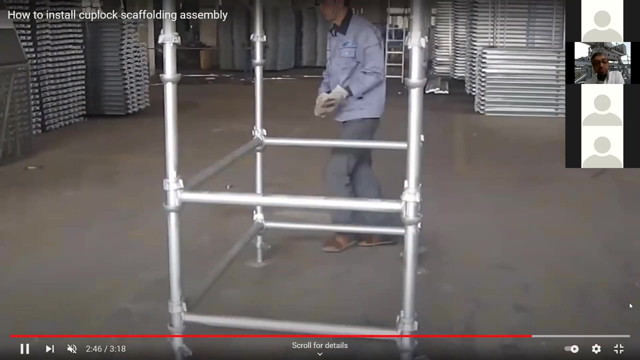 Very easy to fix. Within a few minutes it will be ready. So this can be used as an access scaffolding or it can be used as a shoring to support slabs or beams like that. Okay, So this is basically for access scaffolding with steel planks. 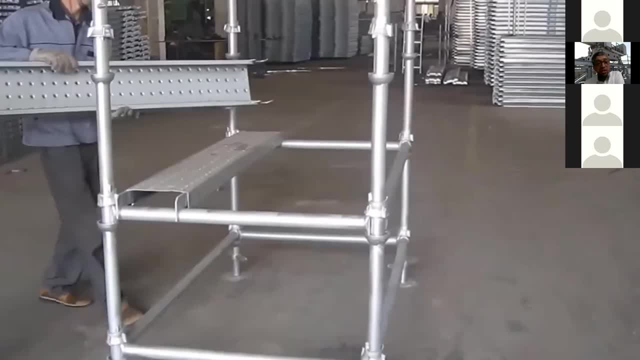 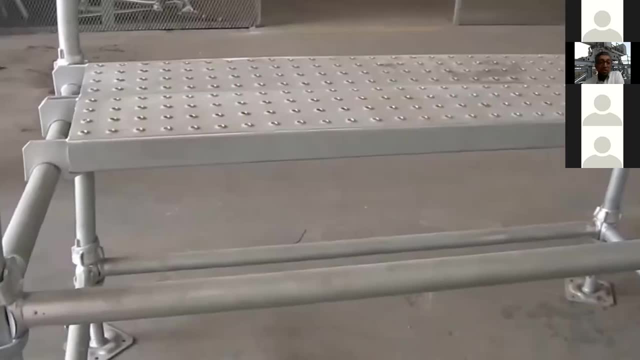 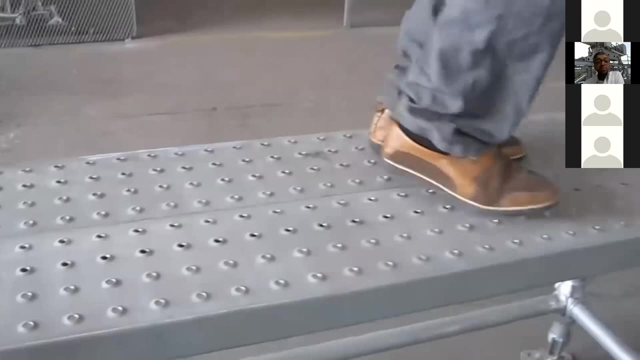 These steel planks also we manufacture. This can be timber also. So, based on the area, if it's working, if we need more fire safety requirement and all we need to go with steel planks And steel planks. it is perforated holes which is perforated. 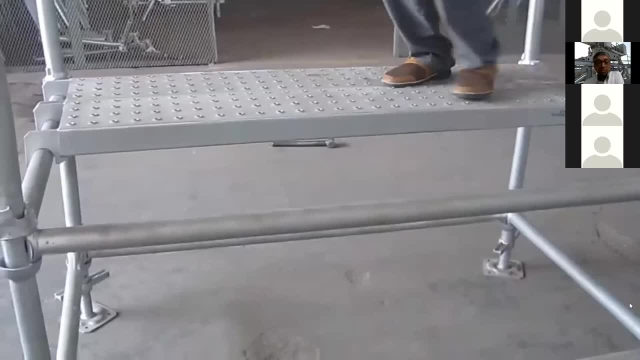 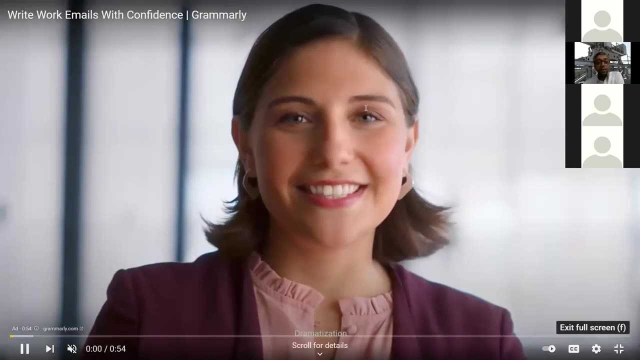 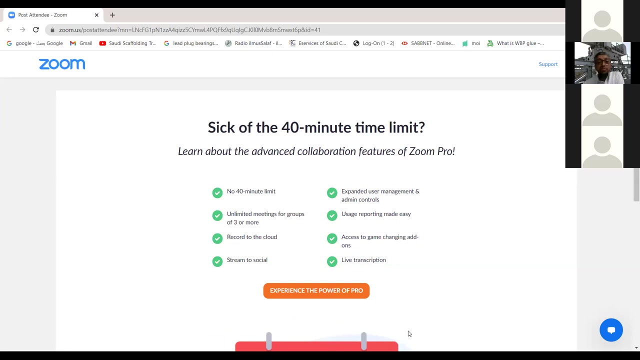 It's protruding out for grips so that you won't slip also. So all this thing you can see. So back to the slide. Can you see the slide? Not yet. Yeah, It's okay now. Okay, Okay, Okay. 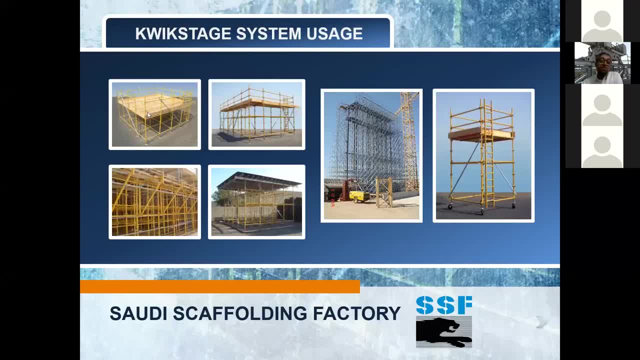 Like that. you can form different types of structures. As I said, there is birdcage, there is independent run, there is shoring system, there is birdcage for some simulation. there is mobile tower. You can put a wheel on the bottom. it will be mobile, like that. 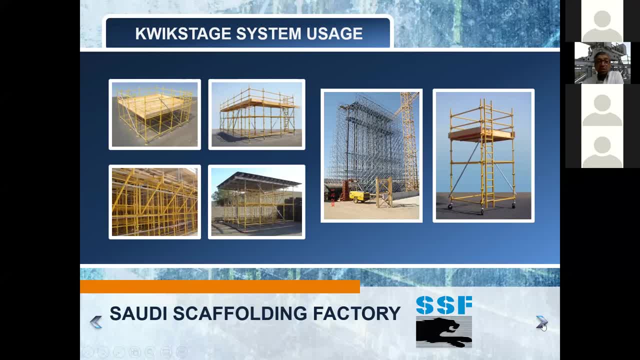 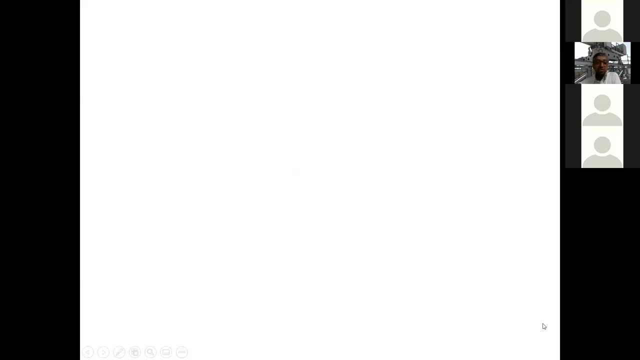 So this is one stage called this is one sort of system called quick stage system. Okay, So this is three stages. When you saw it on the video, which is the one you know, which is one more popular in the market, which is called cup lock system. 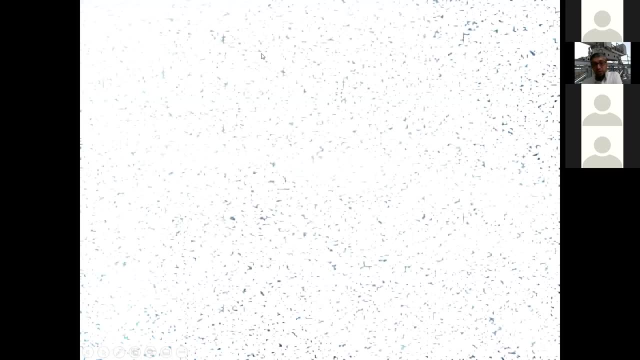 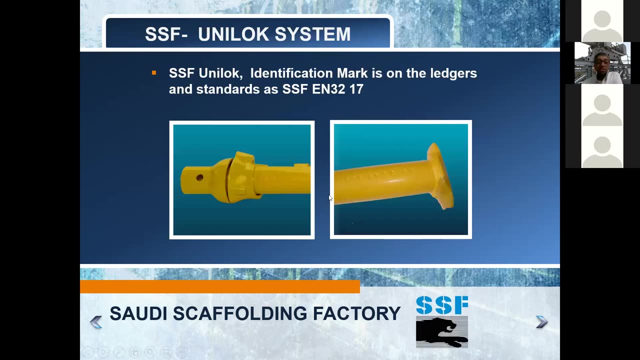 So I'll show you in a minute. Yeah, This is called our SSUP unilock system. This is also Aramco approved. This will look like like this: This is the left one is the standard one, which is having a top cup, bottom cup, which. 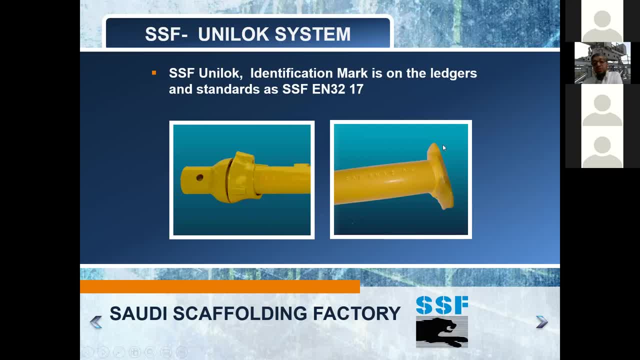 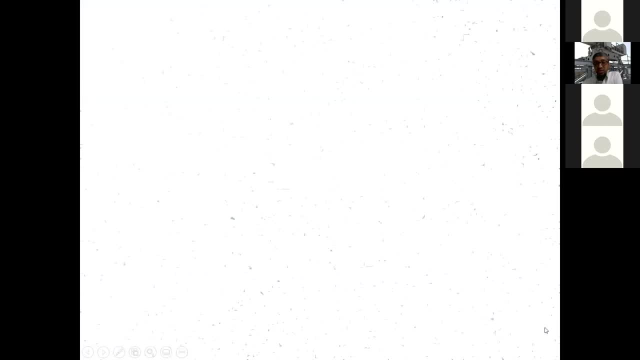 will be staying vertical And this is called the ledger, which is having a blade at the end. Okay, Okay, Okay. So we will go to the next slide. All the specification Aramco has put, specification: it has to match the specification which is: 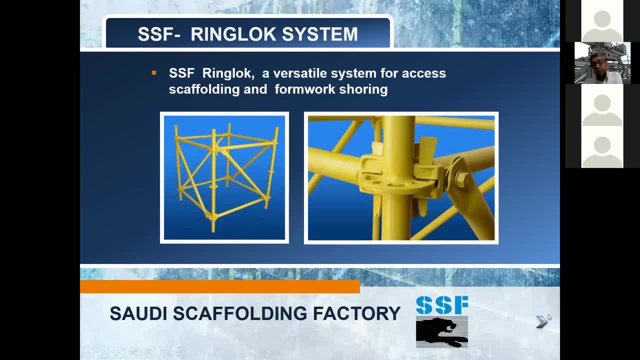 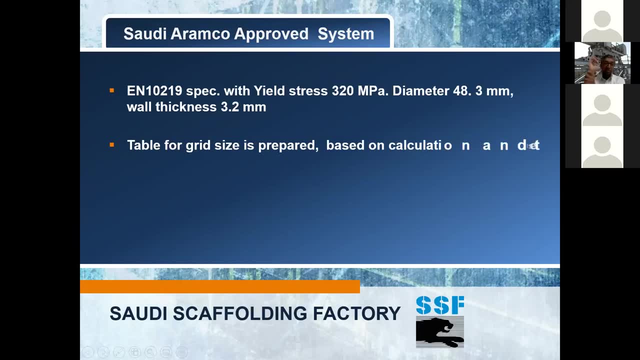 given in their construction safety manual for scaffolding and formwork, which is EN10219, with yield stress minimum 320 like that, And then, based on that, you know, for different, different grid size, we have to prepare testing, We have to do the calculations. 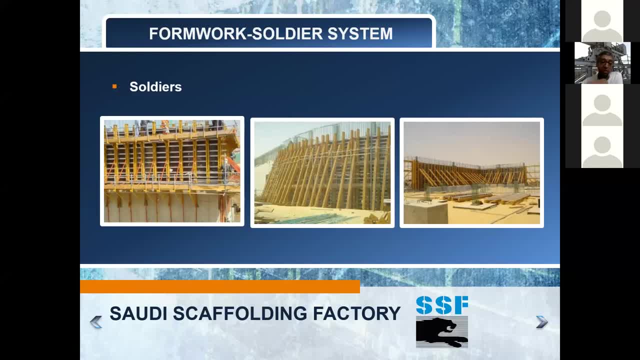 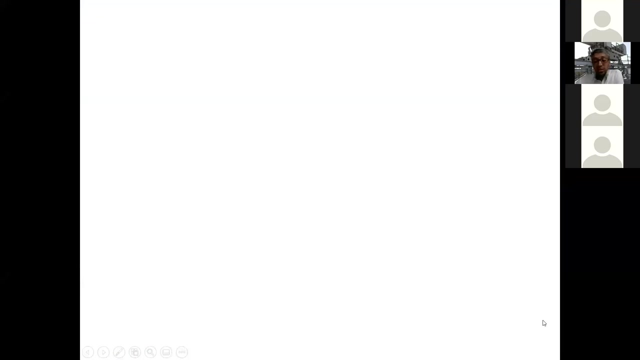 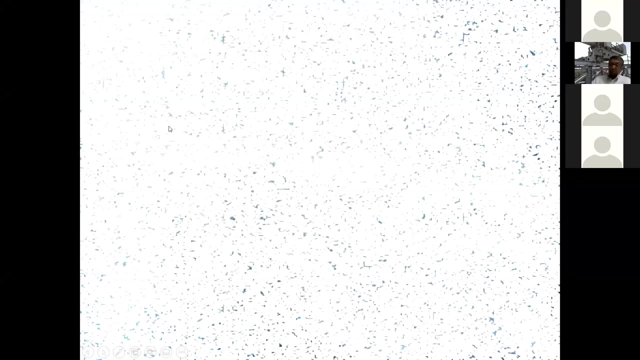 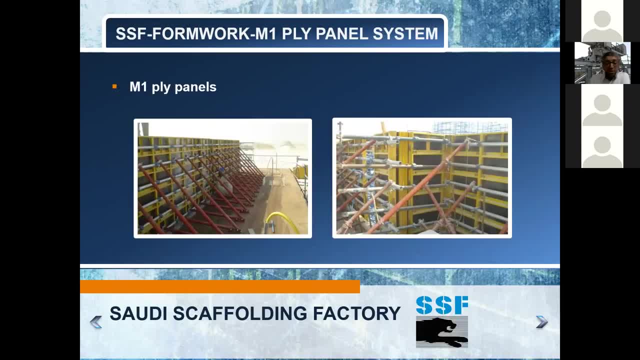 companies near to us, like Aluco. They extrude it and supply to us. This is another system we have which is called panel system. This is again for small wall construction, small foundations. This is a highly versatile system called M1 panel system. This also we manufacture. 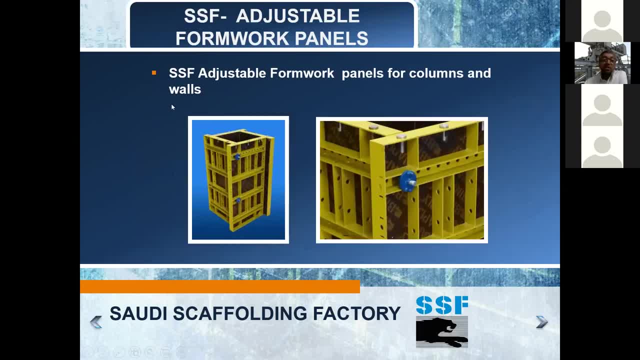 Then we have an improved version of M1 panel system, which is an adjustable panel system, which you know the column size. as you know, in one project you have different size of columns, But you know, with these adjustable panels you can make it to. you know you can. 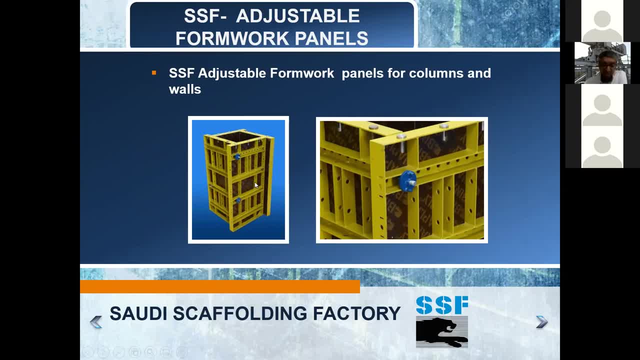 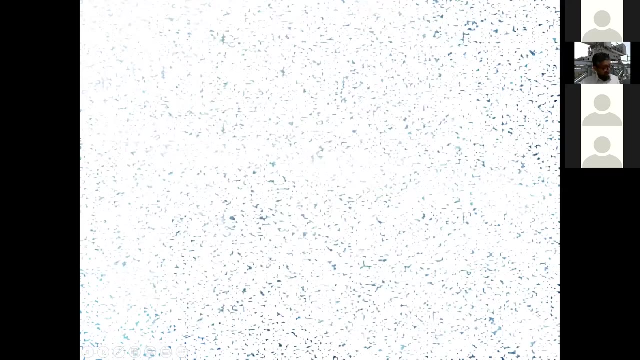 make an adjustment of 5 centimeter of columns. For example, if you use 600 panels, you can use it for 600 to 300 one side. So this is the advantage of this system. Then the other product we have is the tin boiler system. Again, this is channels. 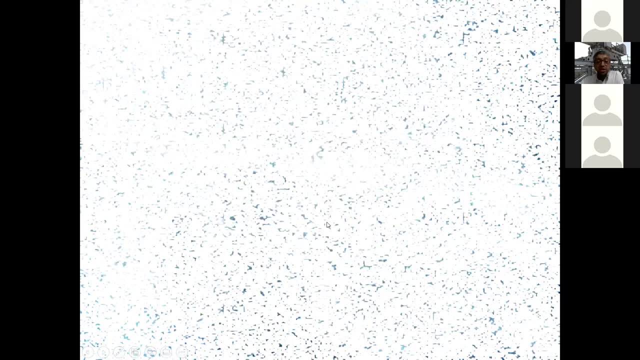 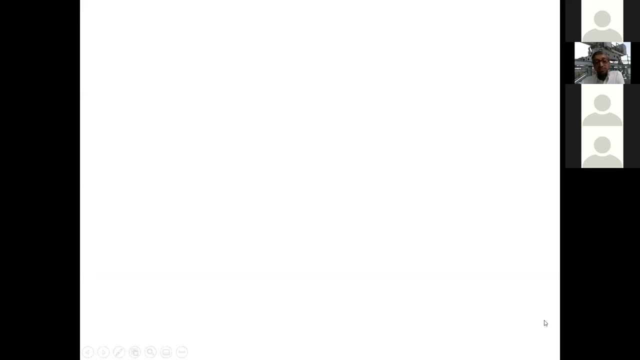 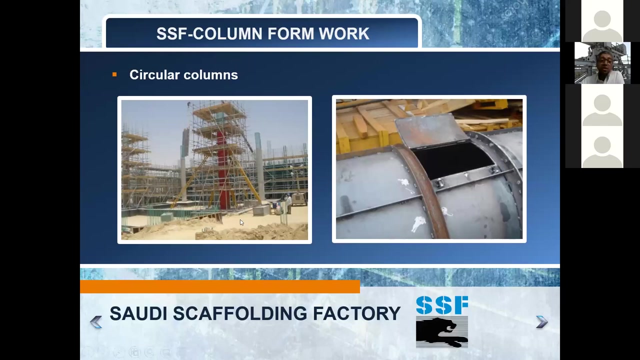 UPN channels, Double back-to-back, you know, which is usually in adjustable panels, which is usually used in column formwork. Also, we have a steel formwork which is completely steel. There is no aluminum involved. Circular: this is a circular column, One meter dia, with 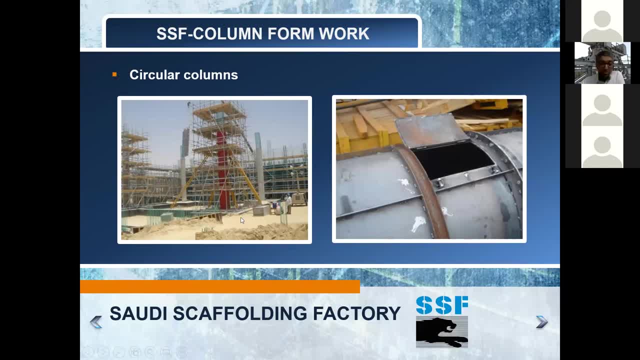 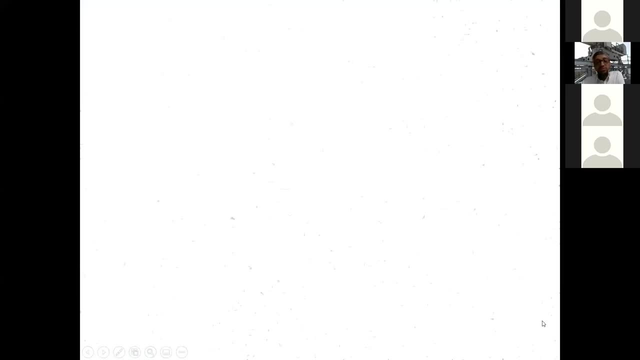 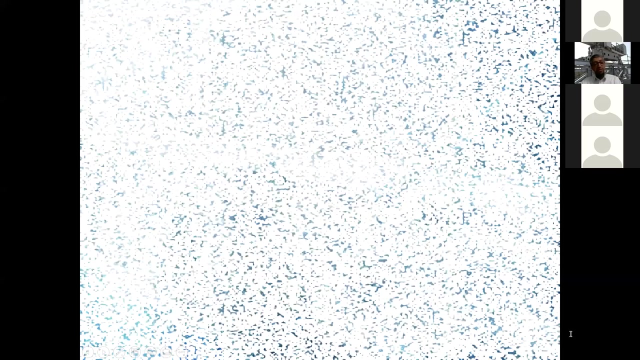 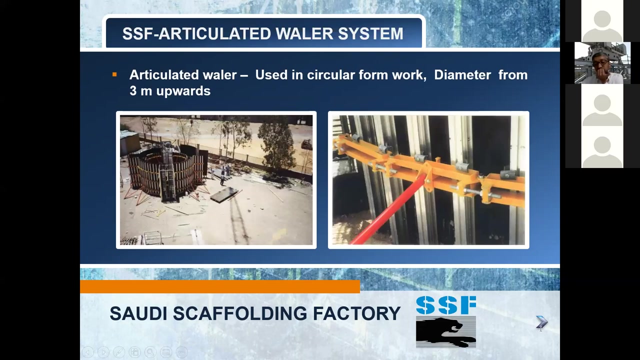 9 meter pore. Again, for this was our project. We have other benefits, like the ó. We have an active ó Which we manufactured in our factory, designed, approved by consultants and, you know, designed and successfully finished. Another important project we did is for the M1 municipality, as the bridge to the two section. 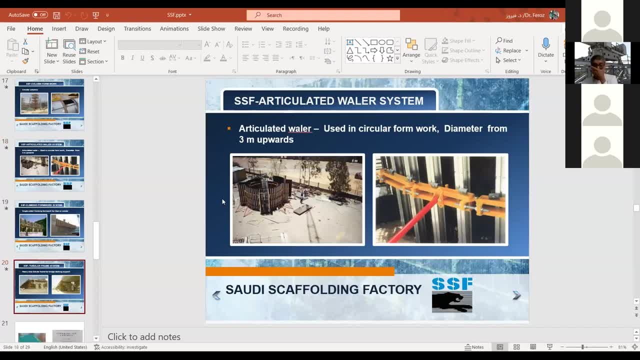 It is a bridge. The other project we did is for the M1 community. We have been doing one of the projects that we have been doing this project for some time here in M1, which, coming across the airport road in the month which he used another system, it's called a framing system. 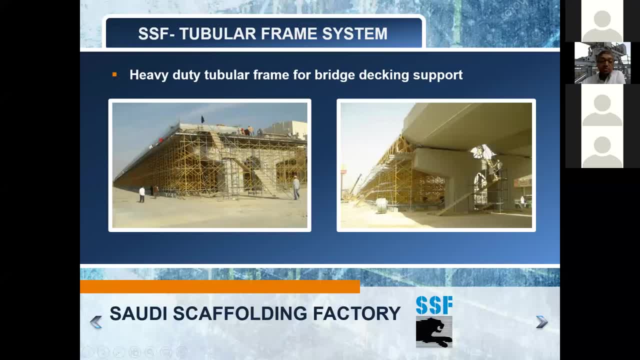 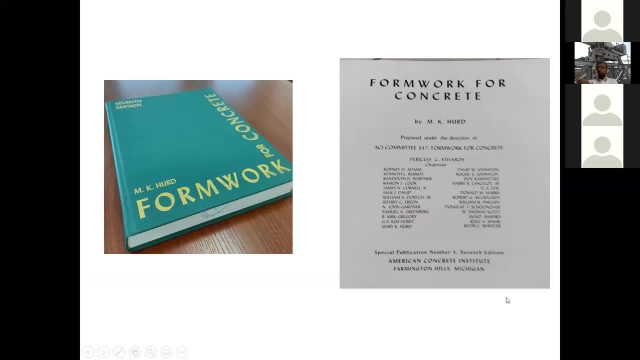 because the loads are very high and the spine of the bridge was so high. so it is a special frame we made for this, for for bridges, and the books and the books we follow for homework. it is this formwork for concrete. uh, this is a very important book for the design, for all the design criteria, so all the 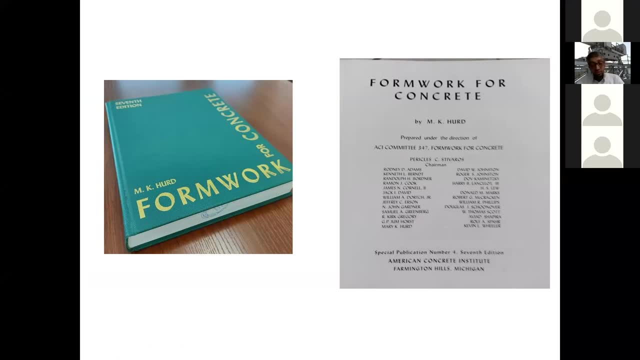 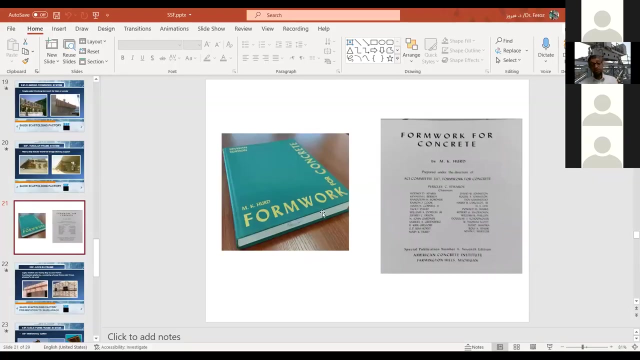 uh, rules and regulations. this will cover all this. again for us, the for for the scaffolding part, we have the construction safety manual from arabco, which are scaffolding and formwork. so basically this is what i was. um no, i want to talk to you about this. 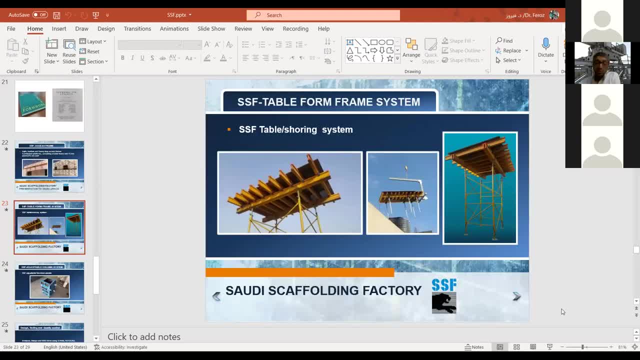 uh, anything, you know this actually. i finished. if you want any additional thing, you can ask. all right, all right, thank you so much, dr firaz. so leave the floor open for any of the participants. if you have a question, you can just kindly raise your hand. yes, is there anyone that has any question? 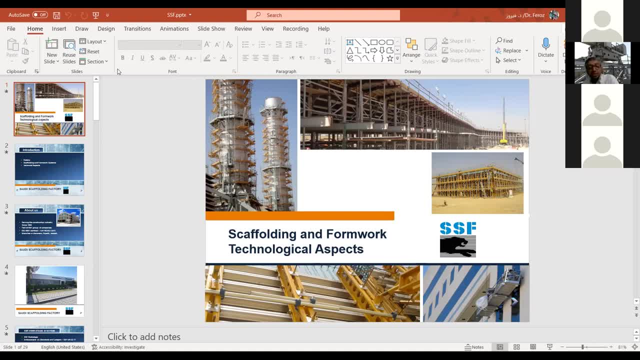 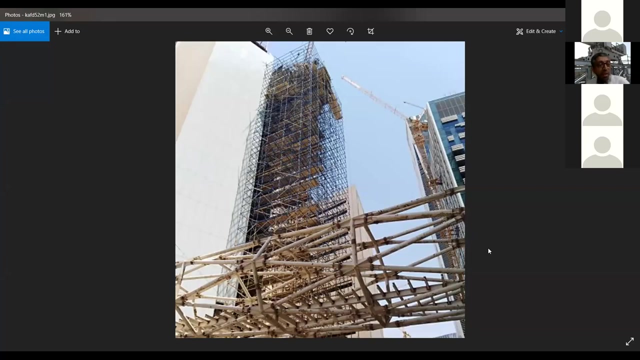 there is. you're welcome. um, um, um. on the safety aspect, you know, as i said, you know there are design criteria. you know, but it's not just the design criteria. you know, in the design of Afghanistan, if you have a need to follow, yeah, and you know we need to submit all the uh certificates if it in a, if it's a. 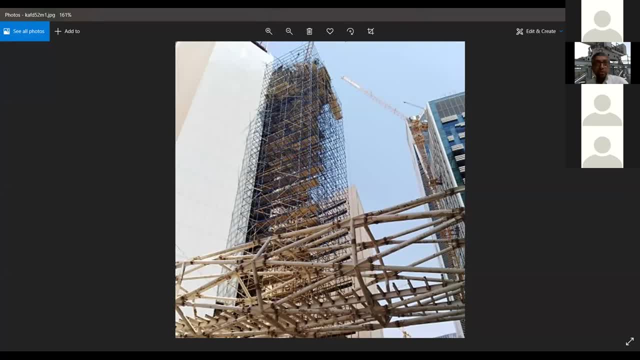 needed. for example, it's a tube. this is mainly tube. no, we need to give a strength of each, each material coming on a regular basis, 40 tons of material, material we buy. you know we need to do one test. this is all as per the specification en10219, as i told you know. 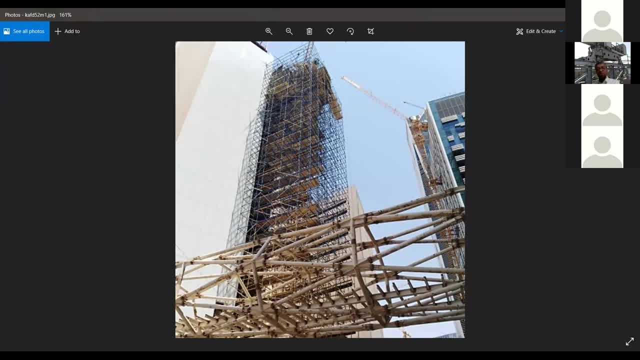 en10219 has specification and aramco construction safety manual also have uh uh specification. so we need to go as per that. then, uh, the third party, like aramco, has the third party consultant, approved consultant. they will verify it. if they have doubts, they will come. 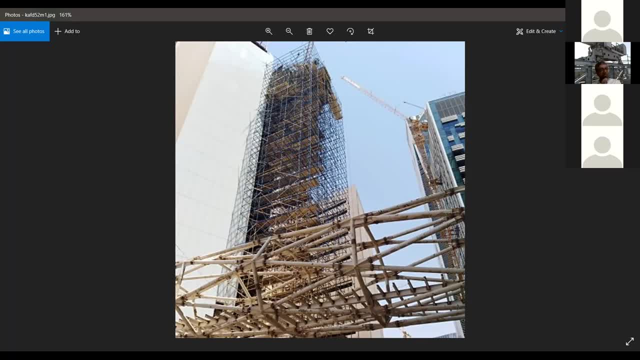 here. they'll need, we need to do testing in front of them, you know. then we need to go there to demonstrate our calculations, design aspects. there are many queries. they'll have comments or thing we need to clarify that, you know. it will take in part, yeah, yeah. so all the, all the. 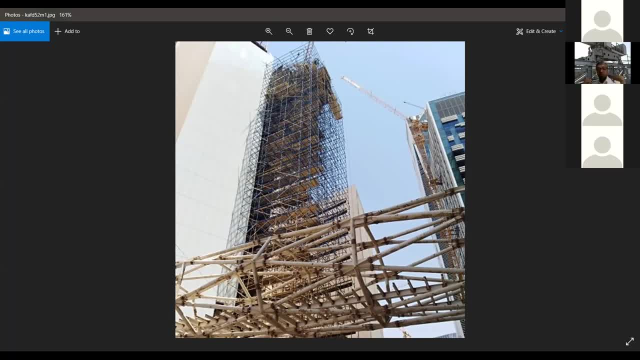 possibilities of unsafety or not comprising to the standards will minimize. okay, okay, excellent, uh. regarding the issue of uh, for example, the stability of this, because i can see here you have a very tall uh scaffolding system. this is how many meters? this is 60 meters. wow, 60 meters. 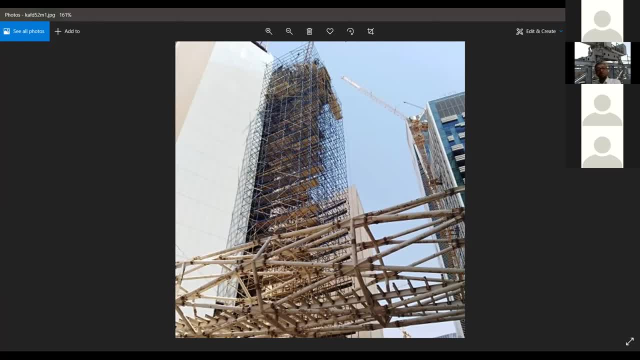 that's almost 20 stories. yes, yes, so like this one. there is a king abdullah finance district in riyadh. okay, kfd, yeah, in this one. now, for example, how do you deal with the issues of stability? you have a lot of wind loads, i believe in in riyadh. we need to, you know, we need to analyze for these strong. 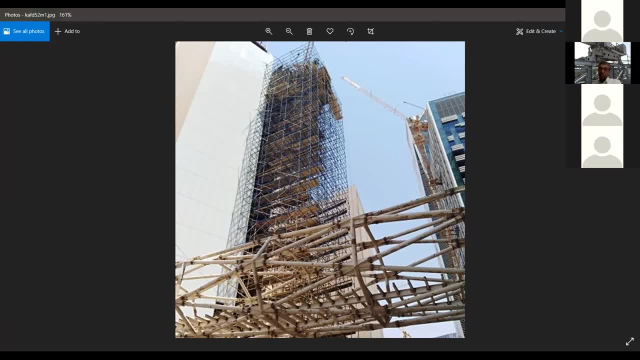 structures. you know we need to because it's outside. i know we need to analyze for wind analysis. then you know, because we are. the advantage is we have an existing structure, a huge structure. we can tie structure and in addition to that now we have bracings, so this will take care of the. 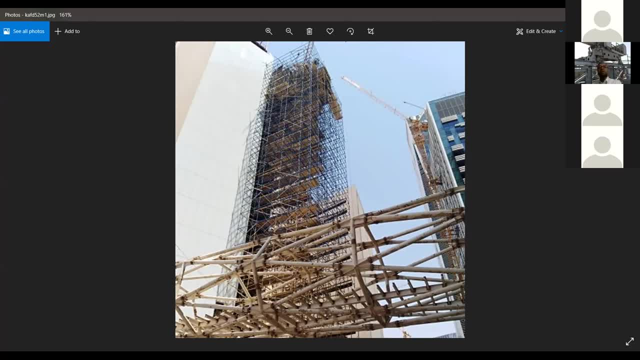 wind load and in all wind acting, it will be uh earthed, or you can say it will be brought down to the ground. yeah, and regarding the breeze, the anchoring, as we said, or brazing, what about to the building? yeah, and for example, do you anchor this uh scaffold to the building? you connect. 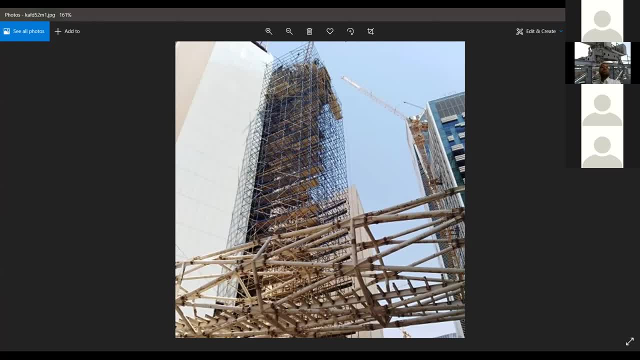 this. we need to anchor it, we need to. this is a very, very important, you know, important- time which is done otherwise. terminology is tying. we need to tie it to the structure, otherwise it will not 60 meter and all you cannot have a freestanding, you know, freestanding maximum. 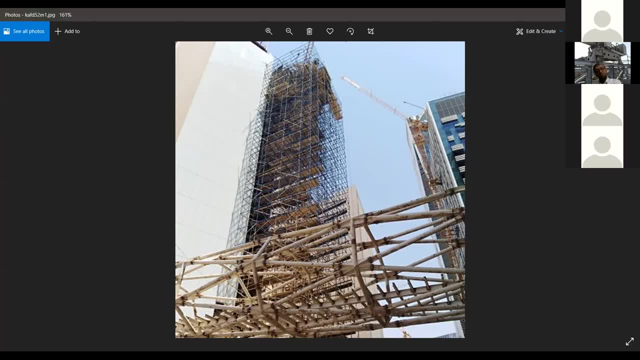 you can have maybe 12 meters only, all right, all right, but even even if you are bracing, it will not okay. otherwise you need to anchor it to the ground. even then it will not work. the lab in a high deflection on the this unknown, you know we do. you know 3d analysis using. you know computer softwares. 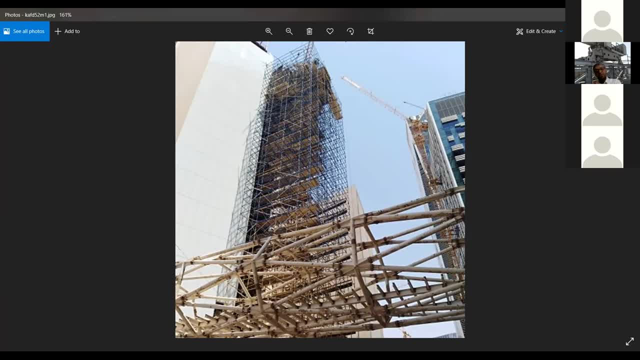 all right. thank you so much, dr. anyone else? do you have any questions, toy? if you don't have any questions, i guess we let dr firaz to call it today. thank you so much, dr firaz. i think i have one comment. yeah, so if somebody asks the question he said: are there specific workers to build the scaffold? yeah, and it. 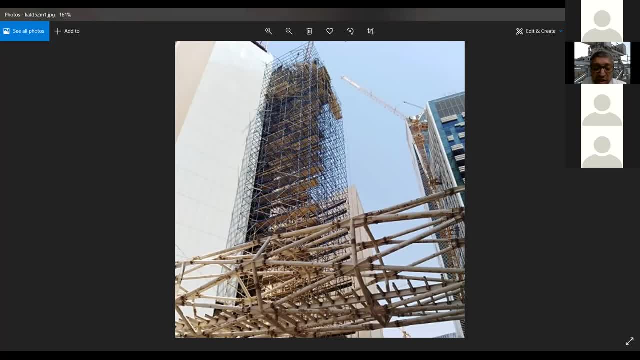 depends on the specip th here don't have any specific mata people to do the construction of the scaffold. do they have any specific training or specific requirements? yes, yes, yes, there is specific training training people, also based in the month. you know they'll, uh, they'll train you for four days, like that. then you'll become a scaffolding inspector or scaffolding erectors. you is also a company in. 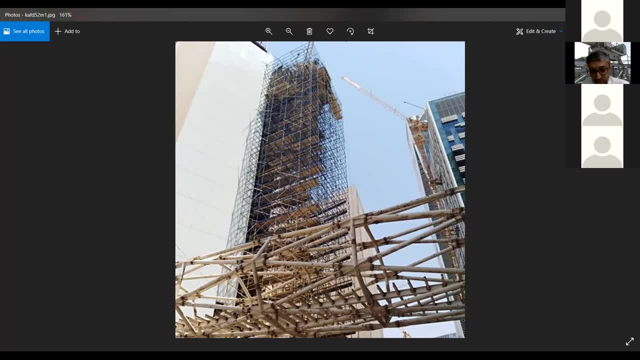 that you need to work on firms like this to know more about the design features of the becomes later. you know there are special training for that, but I i crash their like this to know more about the design, basically civil engineer, civil structural engineering, structural analysis engineering, mechanics engineering, drawings- then only you will be. 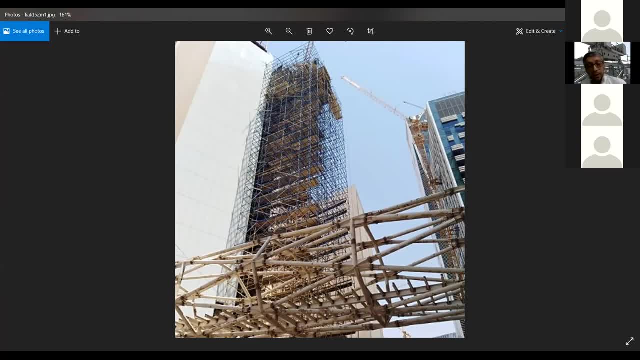 you know, become a good engineer on this type of structure. basically because, as i you know, the basic thing is: this is, after all, it is a steel structure only. yeah, okay, but you know, to specialize it, no, you need to have a basic, uh, understanding of the type of steel structure. then 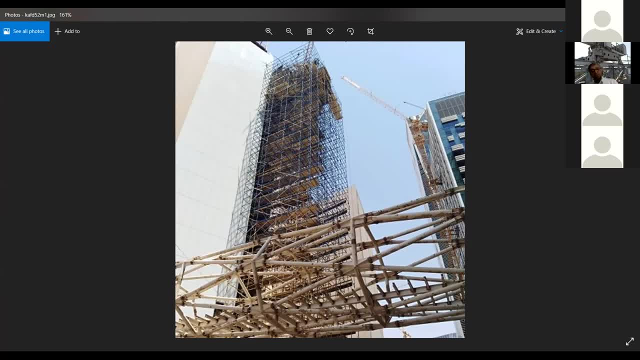 for small uh structures. you know we are training up to 12 meters and they are training in the bomb itself, different uh scaffoldings, but but for tall structures as much as 60 meters and this will require some other specific uh training. yeah, that is more than this one and all you need to.